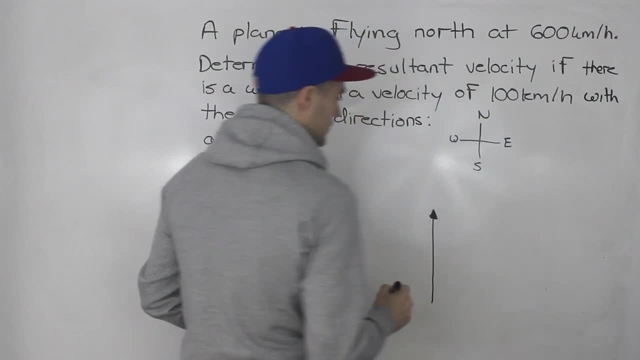 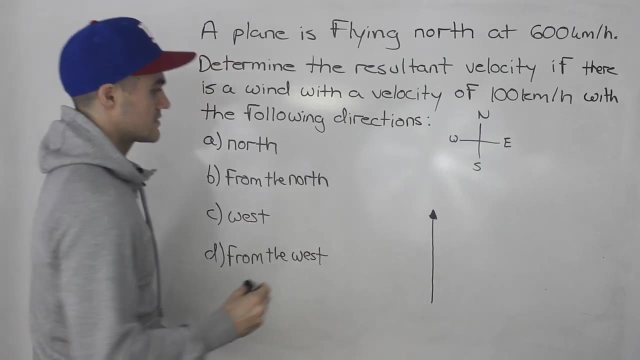 at 600 kilometers per hour. So that is the vector of the plane. And then it encounters a wind. So sorry, let me just label this 600 kilometers per hour. So it encounters a wind with a velocity of 100 kilometers per hour. And then it encounters a wind with a velocity of 100 kilometers per hour. 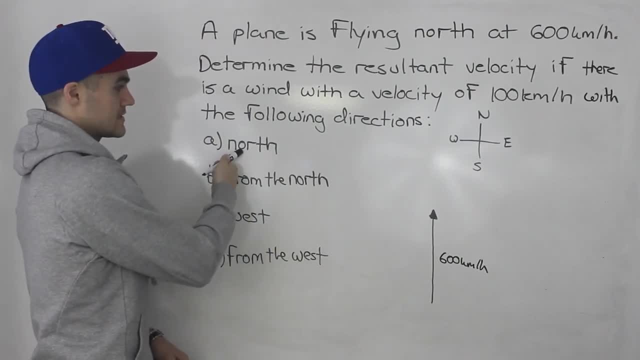 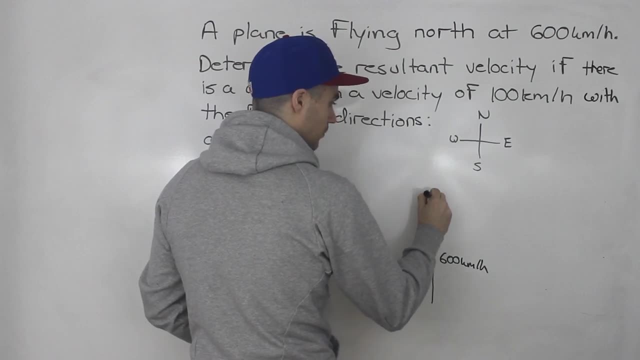 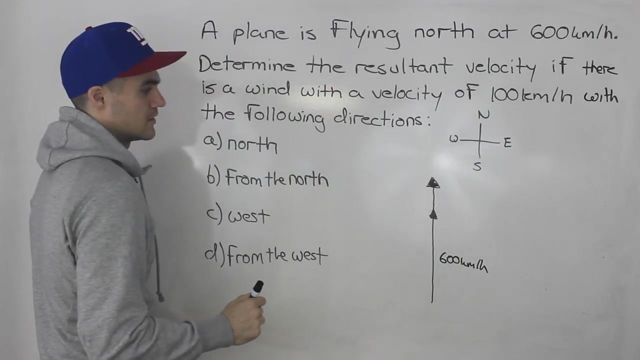 And then it encounters a wind with a velocity of 100 kilometers per hour, And the wind is, in part A, also going north. So what's going to happen? Well, the wind is going to help the plane gain more speed because it's going in the same direction, So you can just add the wind vector right on top. 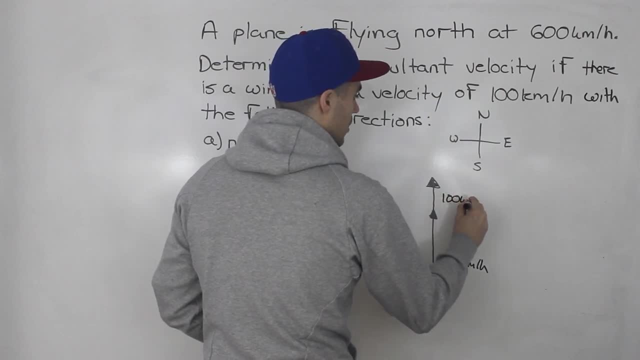 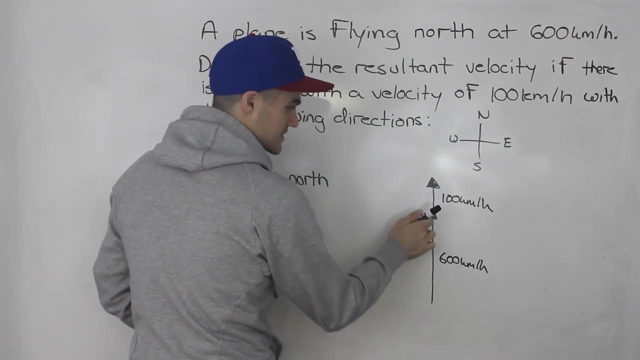 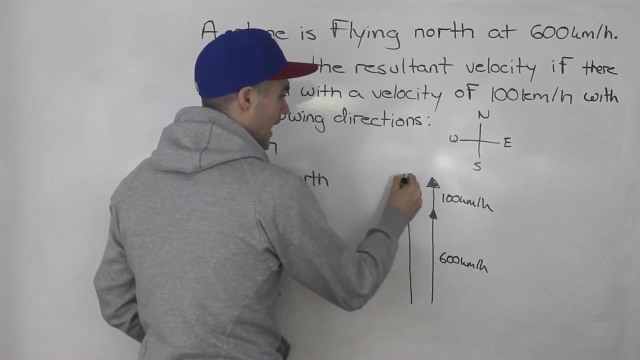 of the plane vector. This wind vector is 100 kilometers per hour. So what's the resultant velocity going to be? Well, with the plane going 600 kilometers per hour, plus the help from the wind of 100 kilometers per hour, it means that the plane is going to be going 700 kilometers. 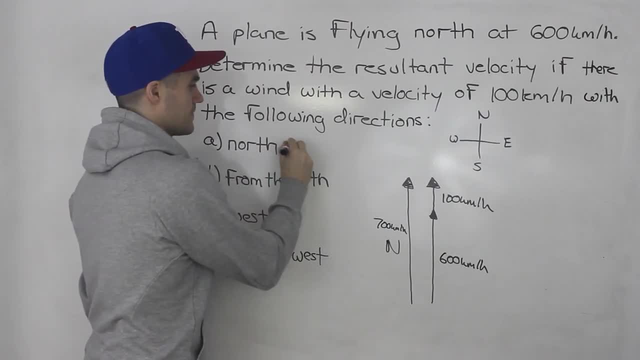 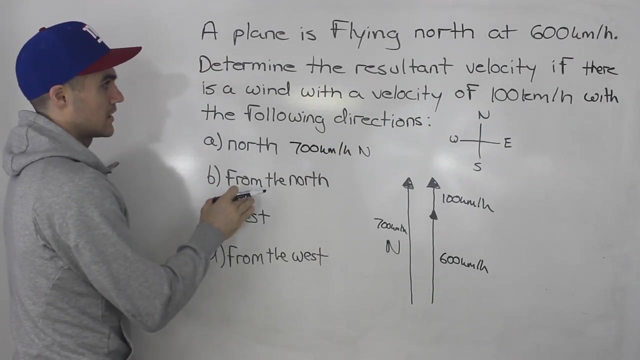 per hour. So the answer for part A: the resultant velocity of the plane is 700 kilometers per hour north. Remember, they're asking for a velocity, So you got to have the speed and the direction as well. Now, what about part B? What if the wind is coming from the north? And that's one thing you got to. 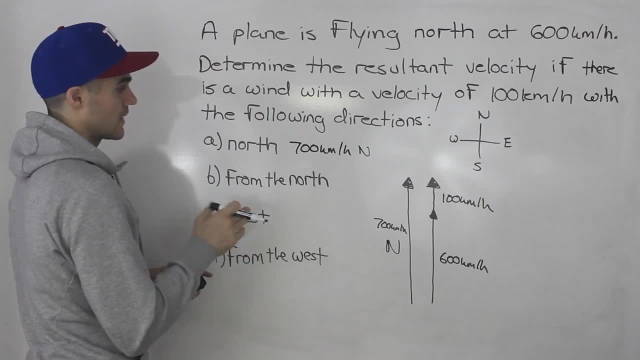 start realizing in these questions. Sometimes they'll give you the direction at which the wind is going, Like in part A, it's going north. Sometimes they'll be telling you it's coming from the north or from a certain direction, And whenever you see that that it's coming, 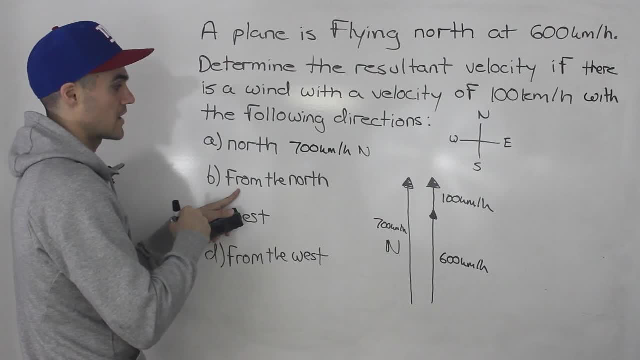 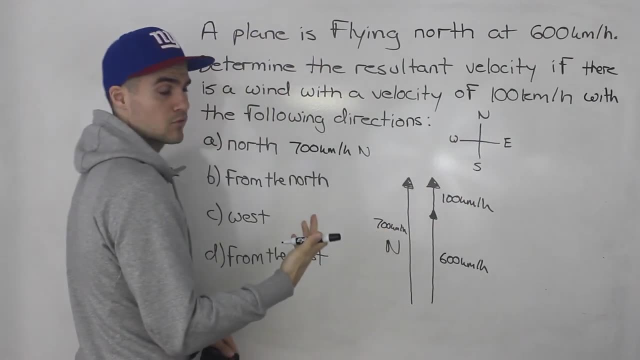 from a certain direction, it just means it's going in the exact opposite direction. So if a wind is coming from the north, then what it really means is that it's going in the direction that the wind is: going south: Coming from the north, going south. So for part B, this: 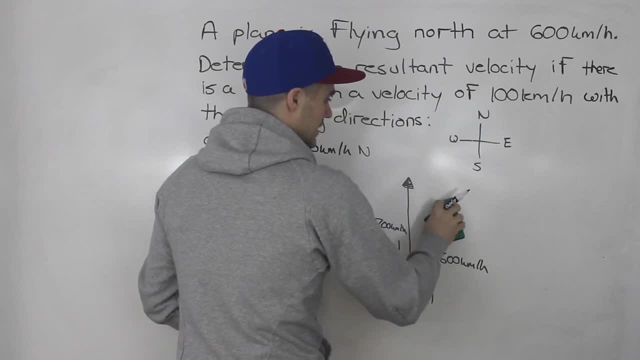 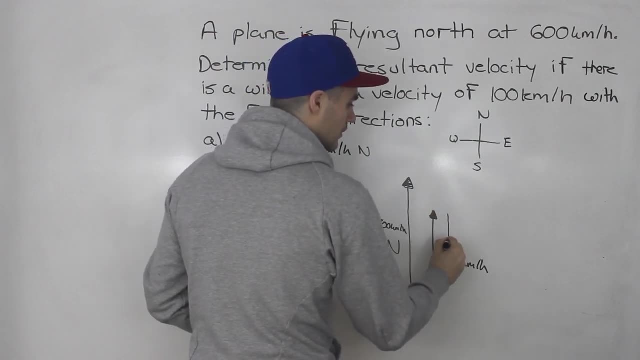 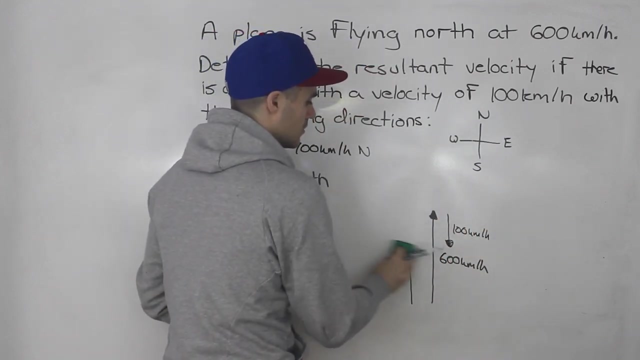 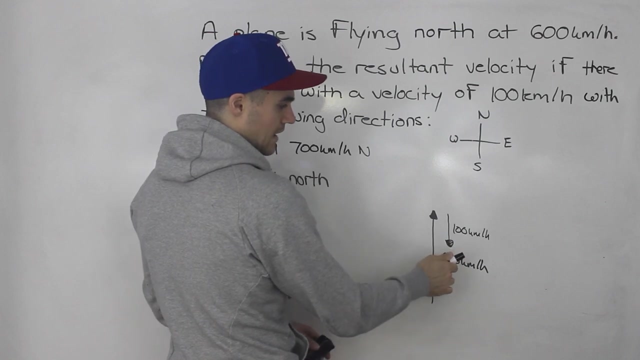 diagram would look different, because the plane is going 600 kilometers per hour north still, but the wind now is going 100 kilometers per hour south, the opposite direction. So what's the resultant velocity going to be? Well, the resultant velocity: the plane is going north, wind is going south, So the wind is slowing down the plane And it's 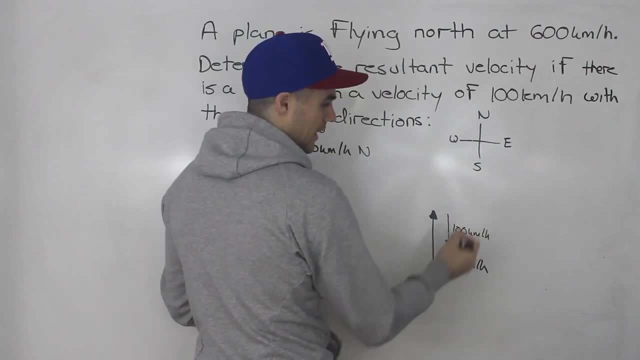 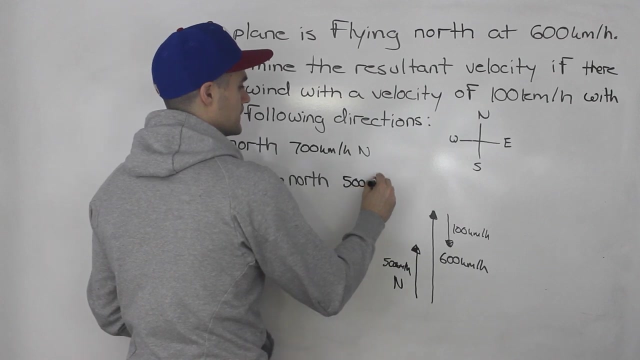 in the exact opposite direction, So it's slowing it down by 100 kilometers per hour. So the resultant: the plane is going to be going 500 kilometers per hour north. That is the answer to part B. Right Plane is going north, but the wind is coming from the north, So it's against it. 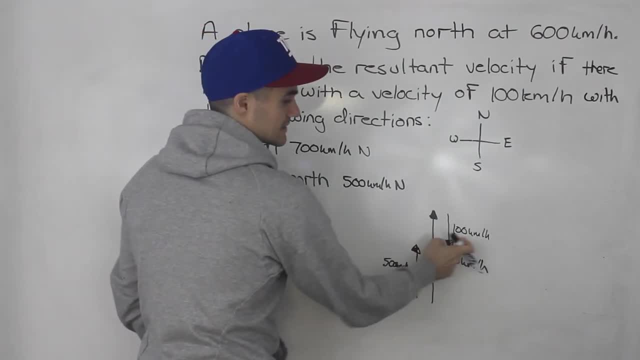 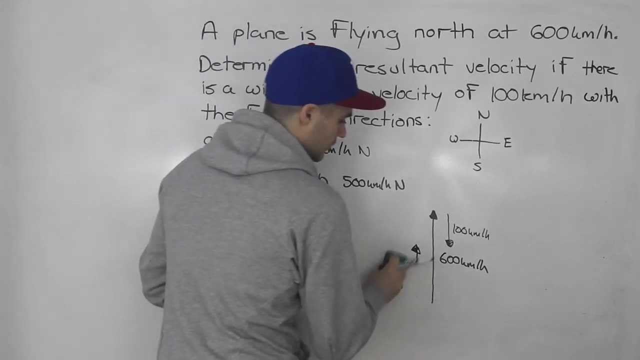 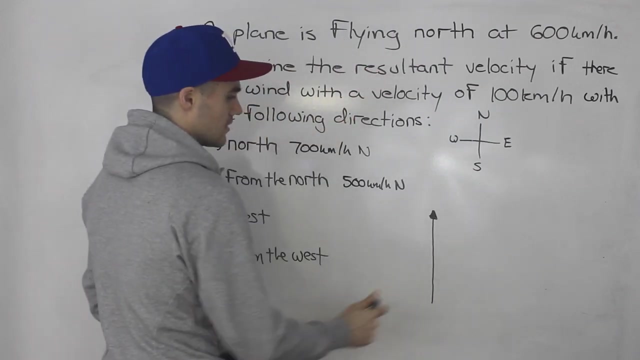 So it's slowing down the plane by that exact speed of the wind because it's in the exact opposite direction. What about part C? What if the wind is blowing west? Well, now it gets a little bit more complex. So this is still the plane. 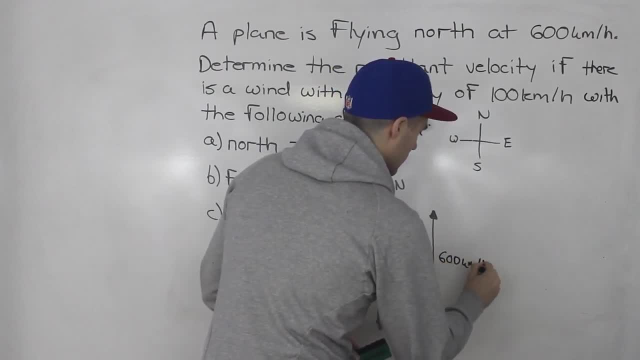 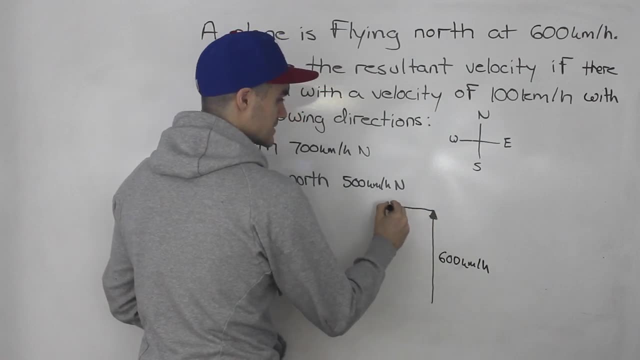 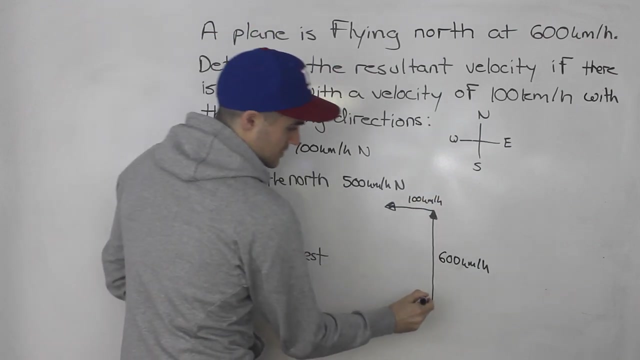 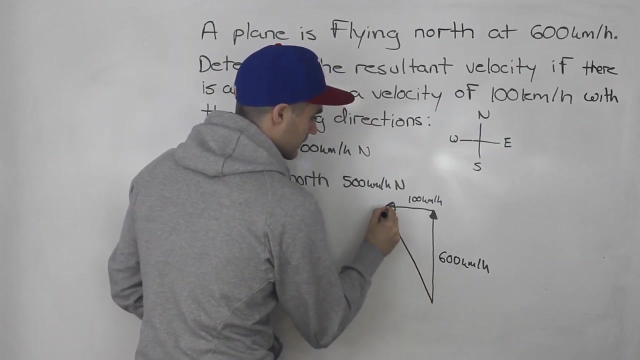 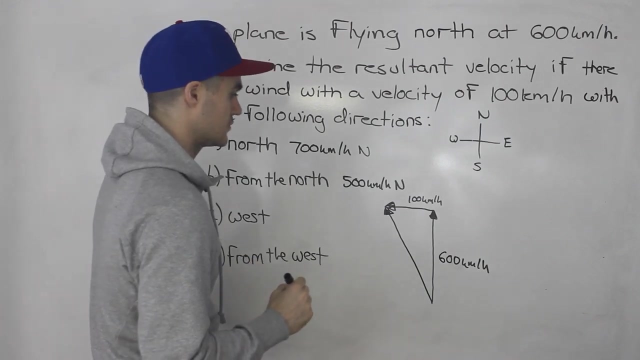 Plane is still going 600 kilometers per hour north, But now it's encountering a wind That is going west, So this is 100 kilometers per hour. So the resultant velocity is going to be from here to here. So now notice, it's a little bit more complex, because what we're going to have to do now 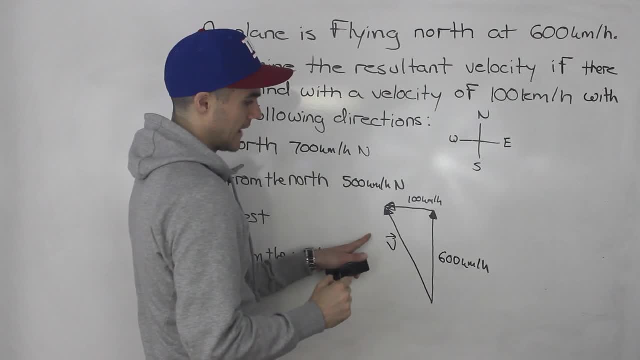 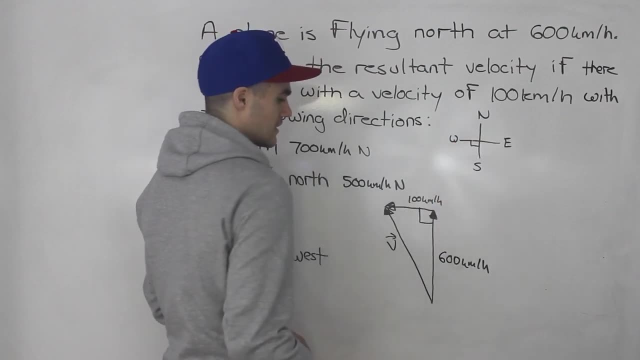 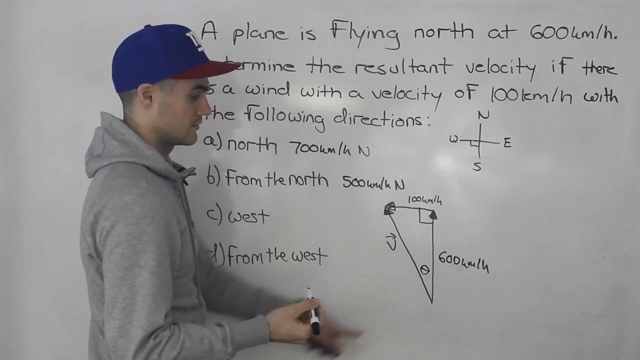 to find this velocity. well, to find the magnitude, we've used Pythagoras theorem: right The right angle triangle, We got north and we got west. That's a perfect 90 degrees right there. And then we're going to have to find this theta here in order to get the direction of the resultant velocity. 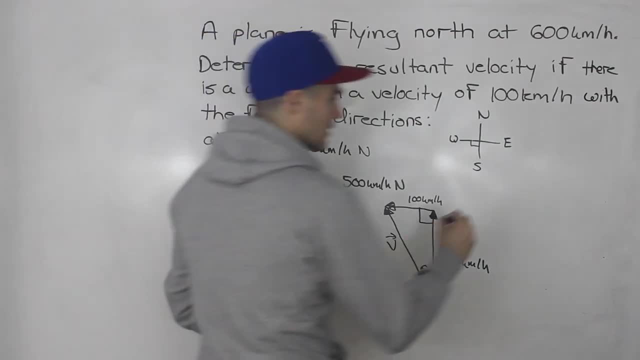 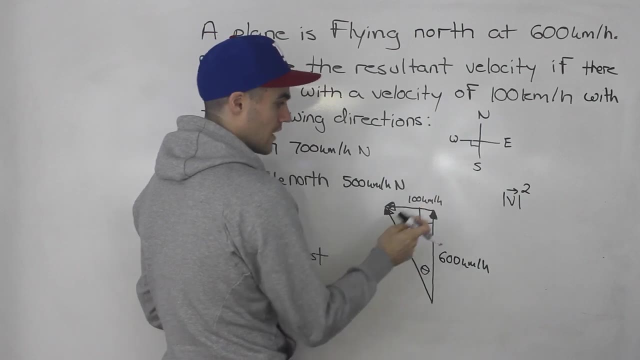 because we can't just get the speed, We've got to have the direction as well. So let's start off by getting the magnitude of that resultant velocity, So we can use Pythagoras theorem. so the hypotenuse squared is equal to 100 squared plus 600.. 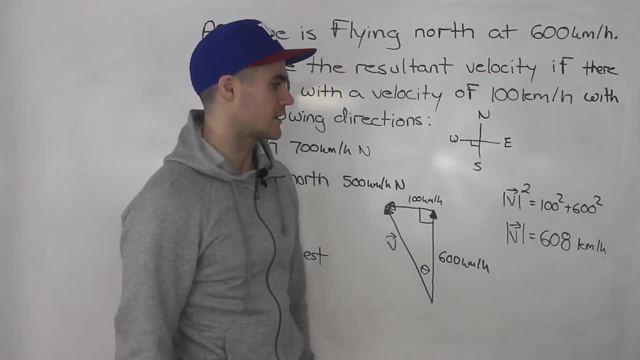 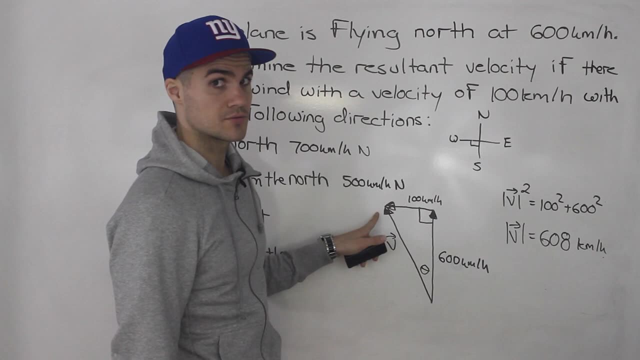 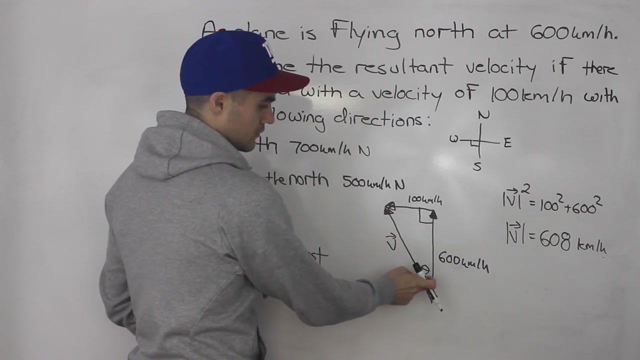 squared, and when you do that calculation you end up getting six hundred and eight kilometers per hour. so that is the speed of the plane, the result in speed, the result in ground speed. we also need the direction. so we got to solve for this theta- notice again, right angle triangle. we can solve for this theta using tan. 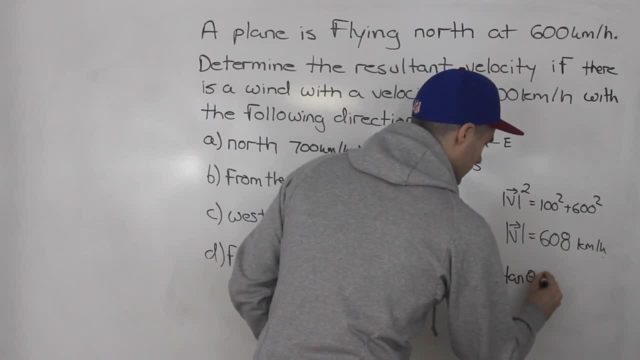 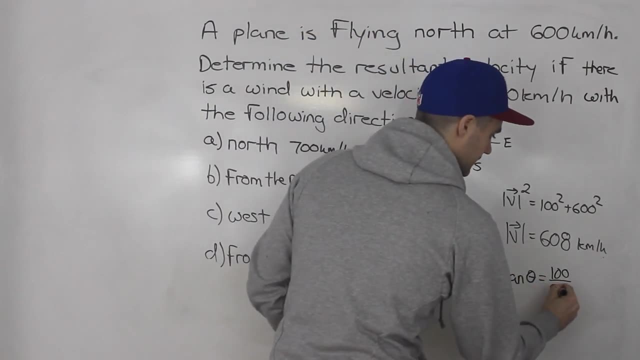 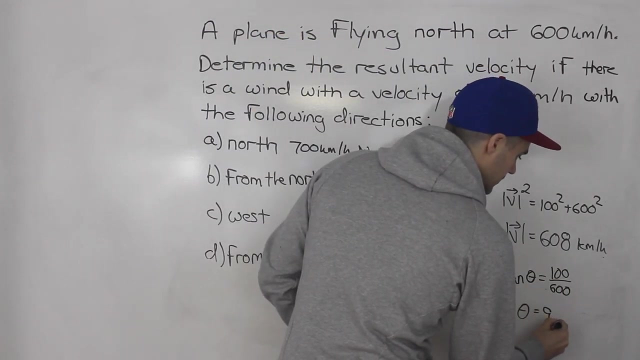 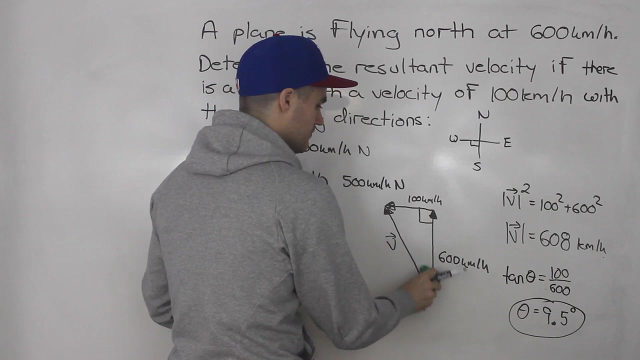 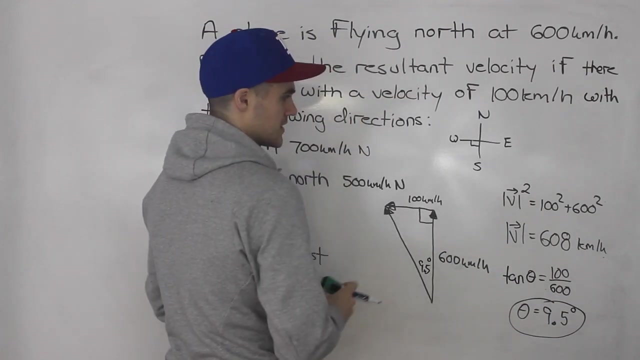 tan of theta is basically the opposite, which is a hundred over the adjacent, which is six hundred, and so when you inverse ten that ratio, you would end up getting approximately nine point five degrees. so this here is nine point five degrees and the speed is six hundred and eight kilometers per hour. 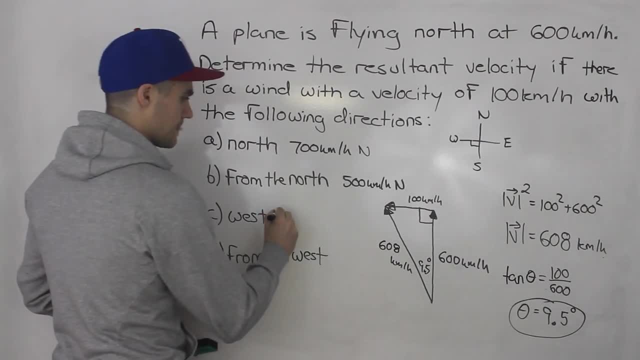 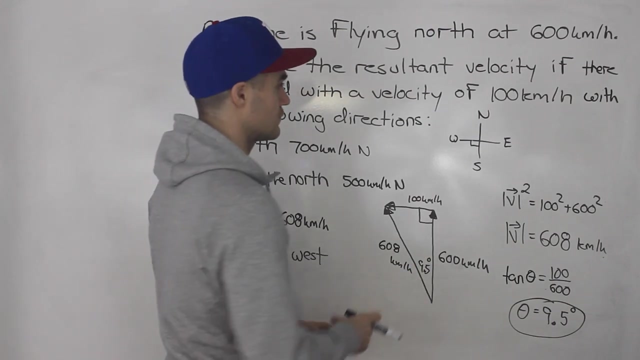 so? so the answer to C is six hundred and eight kilometers per hour. what about the direction? how do we use this nine point five degrees? well, if you think about it, it's nine point five degrees to the left of north. so if we go on this compass, 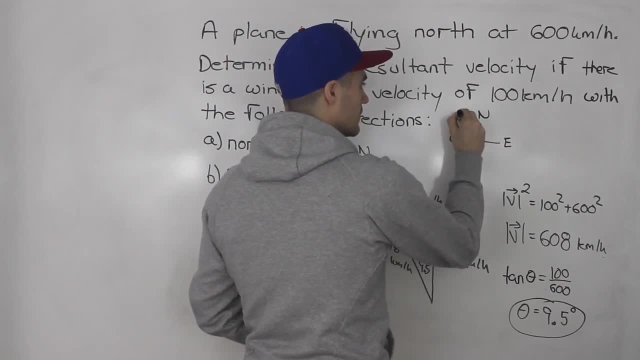 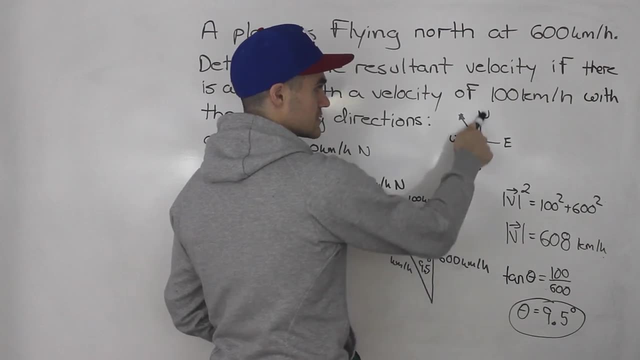 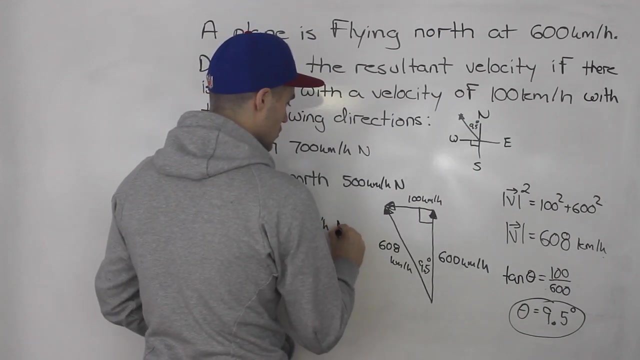 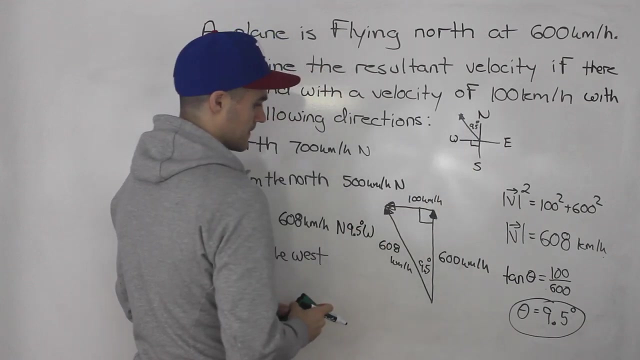 here. basically the plane is going this way and this angle here is nine point five degrees. same thing, because this is north, this is north nine point five degrees to the left. so the way we state that is we say it's north, but nine point five degrees to the west, right so north, but nine point five degrees to the west. and 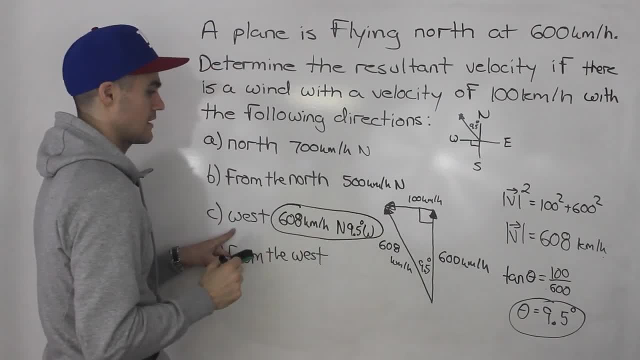 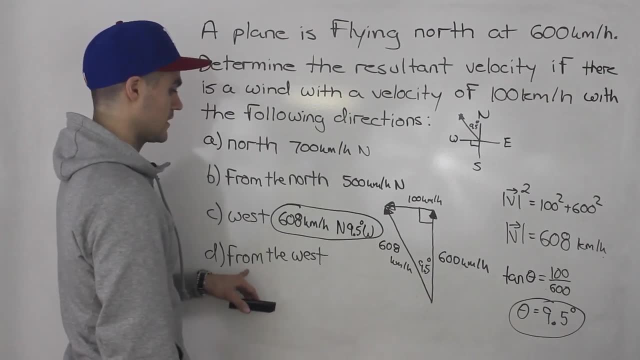 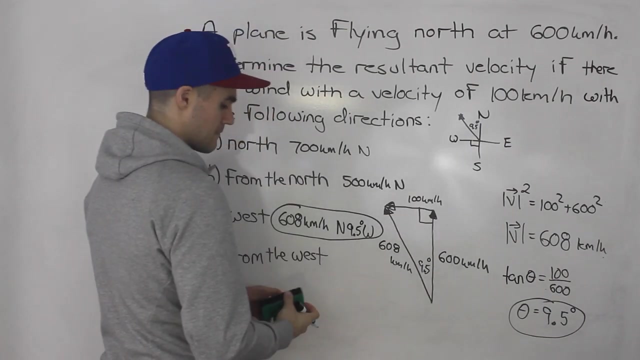 that there is the answer to part C, that is, the velocity of the plane. we got the speed and we have the direction. now what if the wind is blowing from the west? so it's not going towards the west, it's blowing from the west. well, all that. 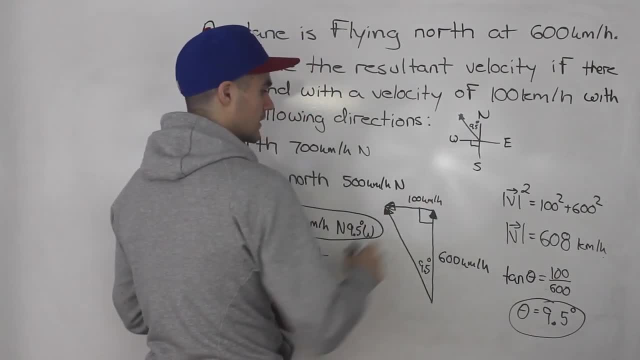 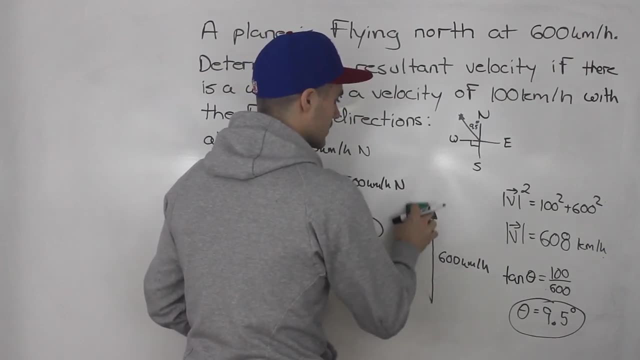 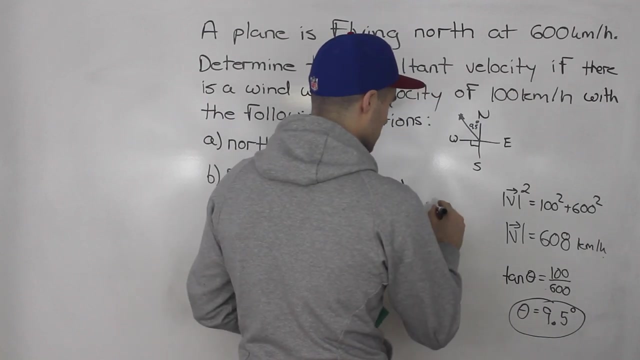 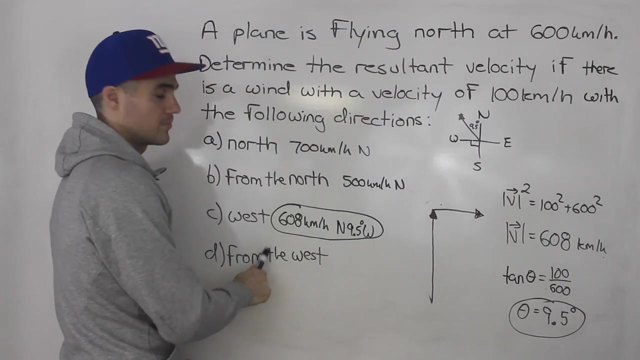 means is that the wind is going to be going in the opposite direction. so, to draw the diagram for that, the plane is still going at six hundred kilometers north. erase this speed as well, because we're going to be going through it. but the wind now is going towards the east right, it's coming from the west.